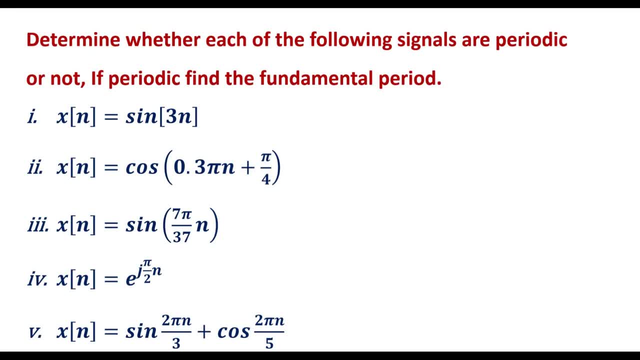 In this video, let me check whether the given signals are periodic or not. Determine whether each of the following signals are periodic or not. If periodic, find the fundamental period. Here five different signals are given. We supposed to calculate, we supposed to verify whether these signals are periodic or not. If periodic, 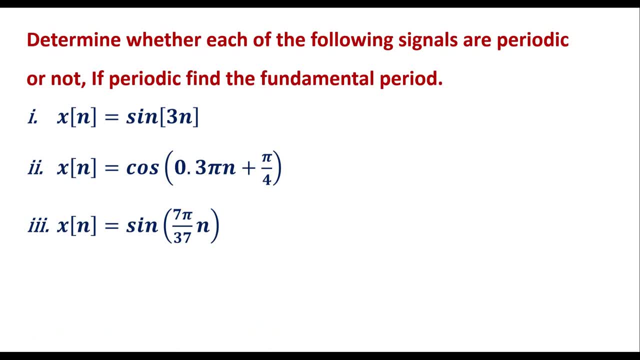 we supposed to find fundamental period? Let me take the first example, That is, x of n is equal to sine 3n. We know that any discrete signal x of n is represented in a standard form as a cos omega 0, n plus 5, where 5 indicates the filled shift. If we compare. this with a 500.. this is a 연verbs restriction. we will have to write 곳 and it has an DIEZ polar LN, A COS, omega 0, N for an alder 1 IN W greed ratio. You can defensively arrive at that in X. 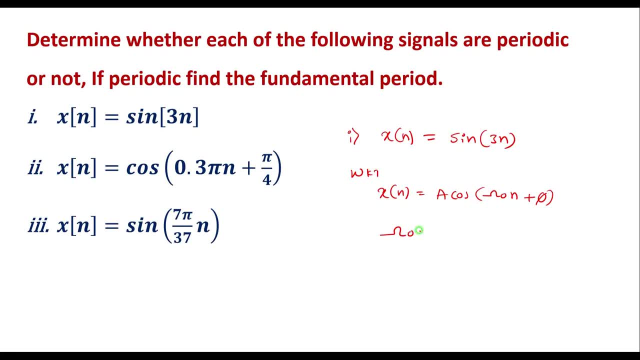 this expression. with this we can say that omega naught is equal to 3.. A discrete signal is said to be periodic if it satisfies the condition. omega naught is equal to 2 pi into m by n. that is so here omega naught, that is, 3, cannot be expressed in terms of 2 pi into m by n. therefore, 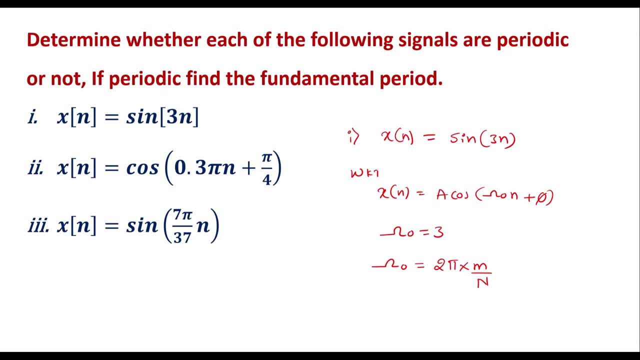 the signal x of n is not periodic or a periodic signal. Omega naught is equal to 3, is not equal to 2 pi into m by n. therefore signal is not periodic. Now let me consider the second example We have. second example is: 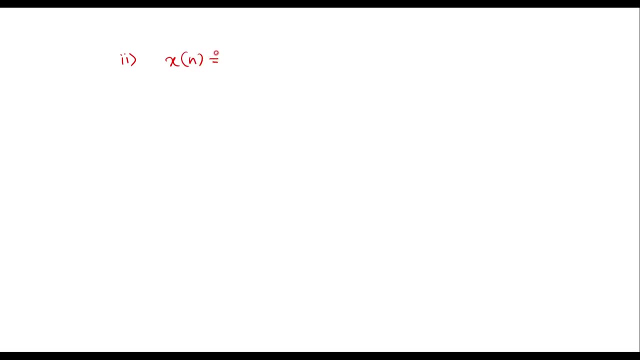 x of n is equal to, we have cos 0.3 pi n plus pi by 4.. So here, if we compare this expression with standard expression, that is this one we have, omega naught is equal to 0.3 pi, where pi by 4 is. 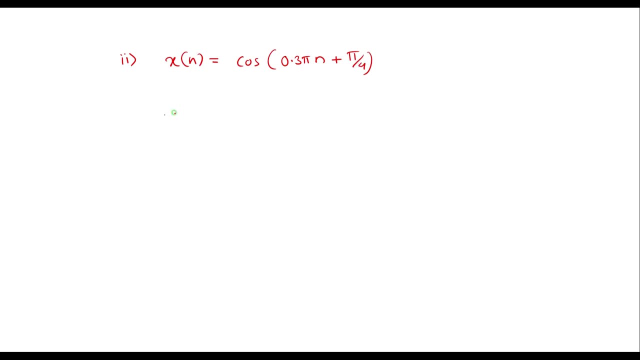 phase shift. We will ignore that phase shift. So here I can say omega naught is equal to 0.3 pi into n. So we are supposed to express omega naught in terms of 2 pi into rational number, that is m by n. So I can represent this 0.3 pi n as omega naught is equal. 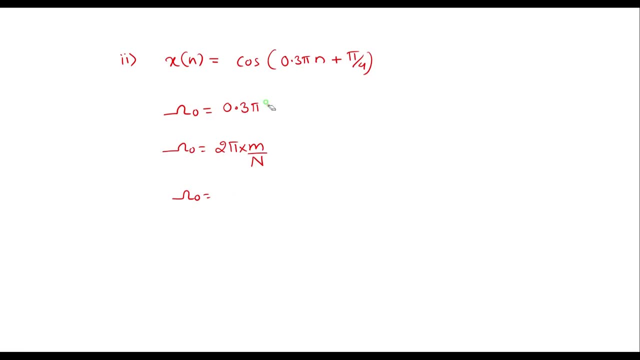 to so 0.3. sorry, this is 0.3 pi. I can represent it as t 3 by 10 into pi, or I can represent this as 2 pi into 3 by 2 into 10, which is same as 3 pi by 10, or I can represent: 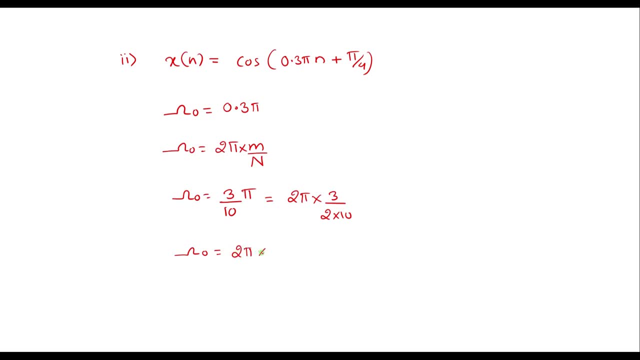 it as omega naught is equal to 2 pi into 3 by 20.. Therefore we can able to express 0.3 pi as 2 pi into 3 by 20.. Therefore the signal is periodic. Therefore signal is periodic And fundamental period is here. n is known as fundamental period. So. 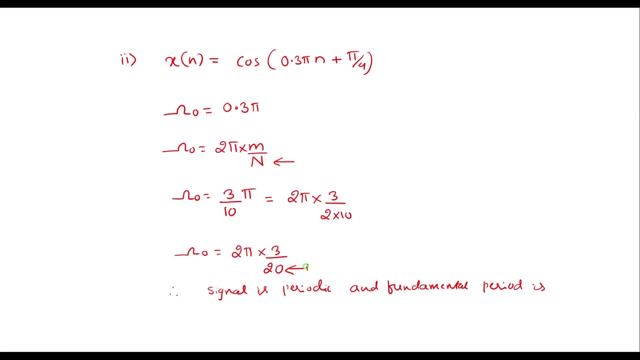 comparing this expression with this. So here n is 20, fundamental period is here n is equal to 20.. Now let me take the third example. Now we have x of n is equal to sine 7 pi by 37 n. So here, if you compare with the standard signal, we 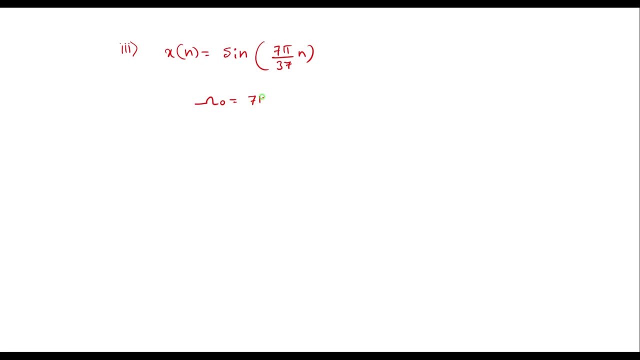 can say that omega naught is equal to 7 pi by 37. So we supposed to express this omega naught in of: omega naught is equal to 2 pi into m by n form, If we are able to express in this form. 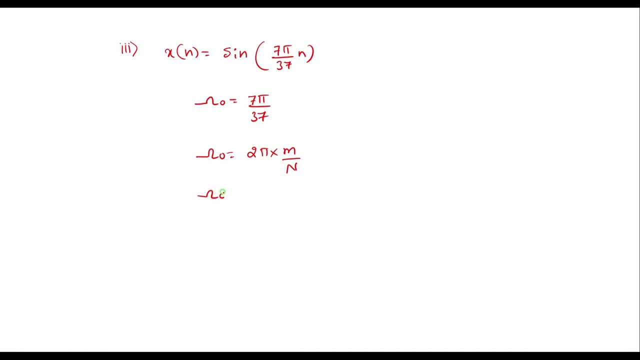 we can say that signal is periodic, So I can represent it as omega. naught is equal to this signal, So I can represent this as 2 pi into 7, by 37 into 2.. That is, if we cancel this 2 and. 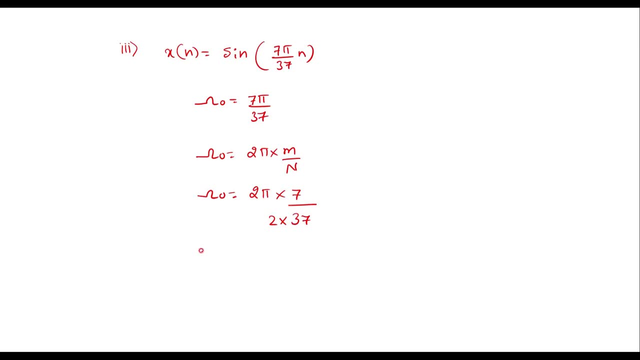 2,, we will get the same thing, that is, 7 pi by 37. So omega naught is equal to 2 pi into 7 by 74. So therefore, signal is periodic and fundamental period is that is fundamental period. n is equal to, that is 74. If you compare with this expression, n is equal to 74.. 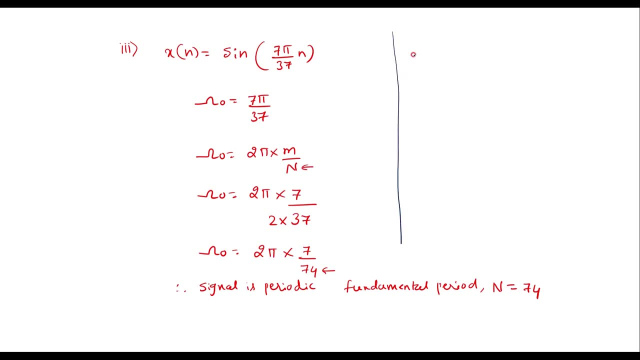 Now let me take the fourth example I will take here, that is, x of n is equal to e power j pi by 2 n. So here it is of form e power j omega naught n. So here omega naught is equal to 2 pi into 7 by 37, into 2 pi into 4.. So here it is of form e power j omega. 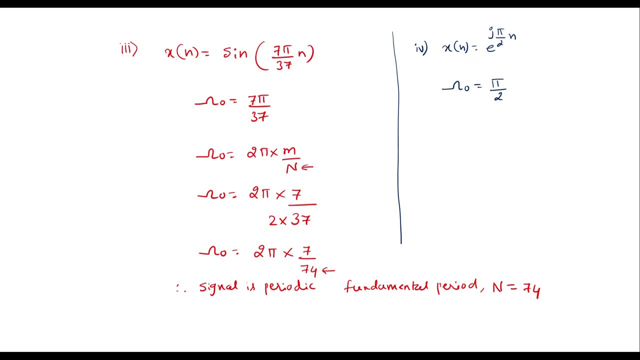 omega naught is equal to pi by 2.. Now we will try to express this omega naught in standard form, that is, omega naught is equal to 2 pi into m by n form. So expressing this pi by 2 in terms of this as: 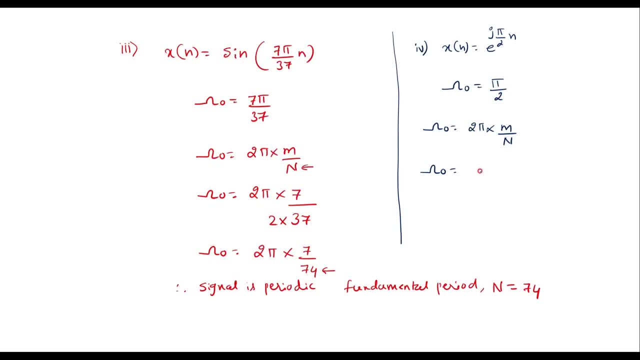 omega naught is equal to here. already we have pi. here we have pi, that is pi into 2.. I will multiply this with 2.. So in denominator, I will multiply the term by 2, that is 1 by 4.. So if we 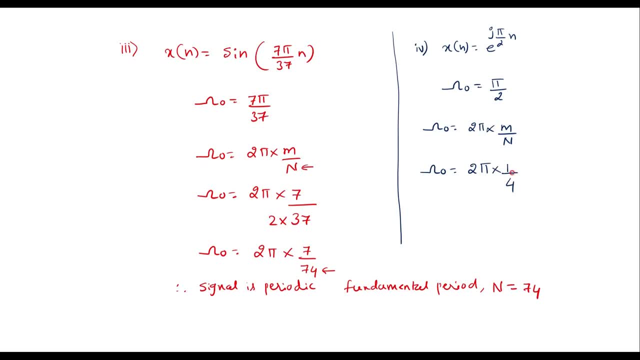 take 2 pi by 4, we will get the same thing, that is, pi by 2.. So this is of form 2 pi into m by n. So here this is n. Therefore this signal is periodic with fundamental period. Frequency. with fundamental period, n is equal to 4.. So let me consider the fifth example. 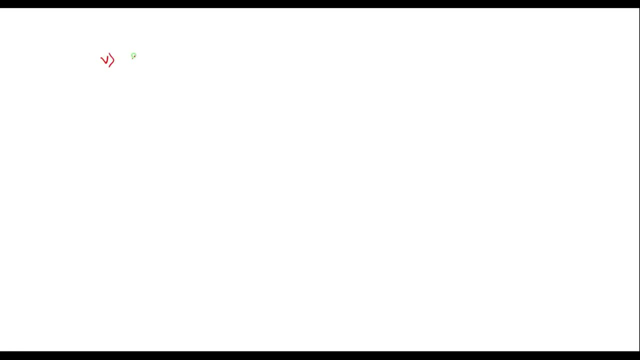 that is, x of n is equal to sine 2 pi by 3 n plus cos 2 pi by 5 n. So here we can see that x of n consists of two signals. So this is called composite signal. It is made of two different signals. So here let me write: omega 1 is equal to, here it is of form. 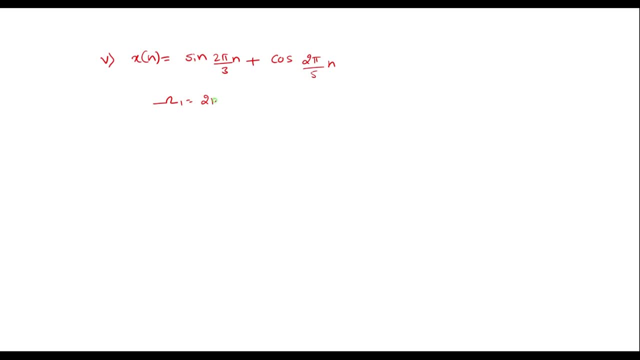 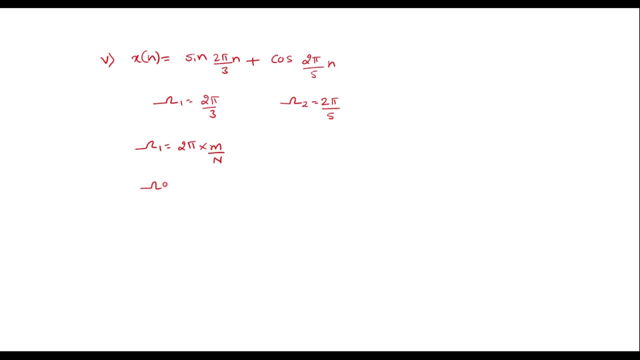 let me write: omega 1 is equal to 2 pi by 5.. So here let me write: omega 1 is equal to 2 pi by 5.. So here m by n, that is, I can represent it as omega 1 is equal to 2 pi into 1 by 3, 1 by 3.. So here I can. 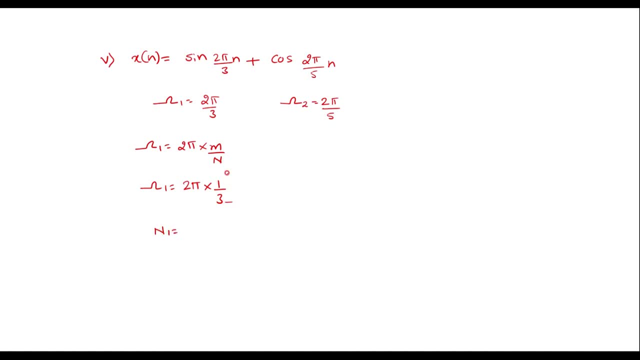 say n1 is equal to, this is: n1 is equal to 3.. Similarly here I can say: omega 2 is equal to 2 pi into m by n2. or I can write: omega 2 is equal to 2 pi into 1 by 5.. Therefore n2 is equal to. 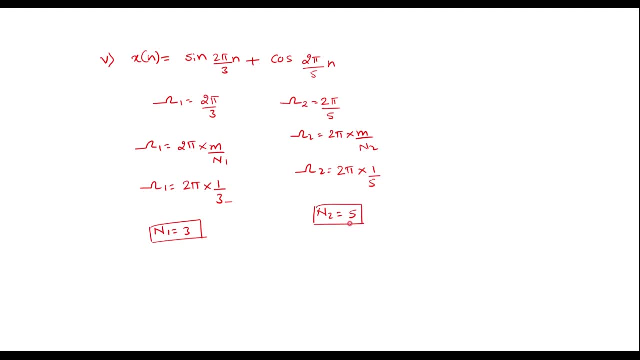 5.. So if we take the ratio of 3 and 5, so in composite signal we are supposed to perform n1 by n2, which is equal to 3 by 5.. So here 3 by 5 is a rational number.